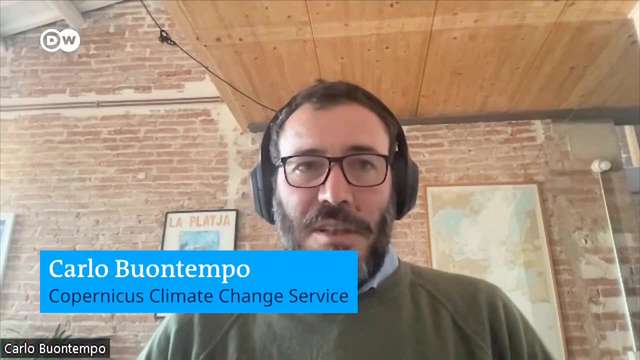 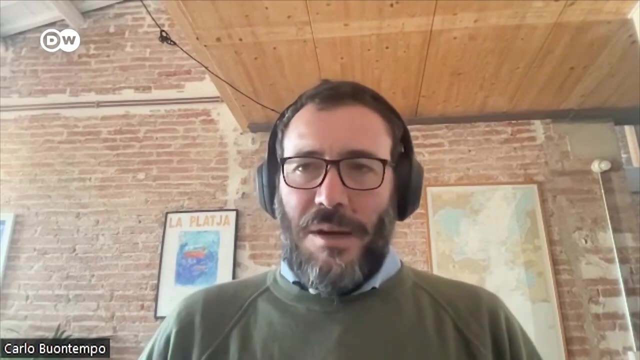 There is this tendency towards higher temperature and this is largely driven by changes in greenhouse gases in the atmosphere. So the CO2 and water vapor and methane. 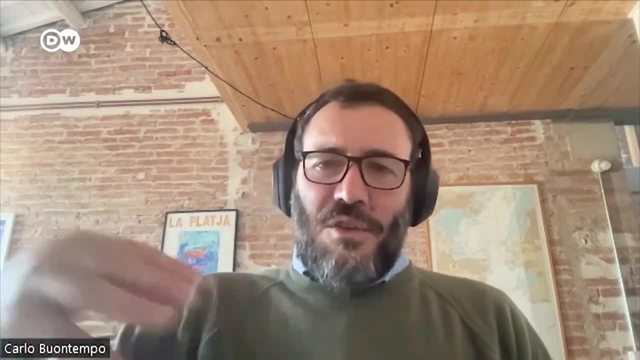 And so on. And this has been the main driver for this constant warming. 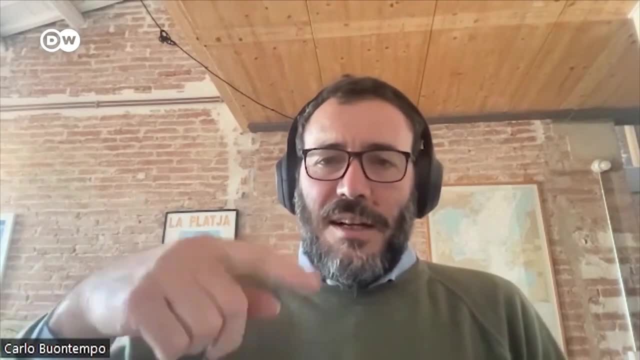 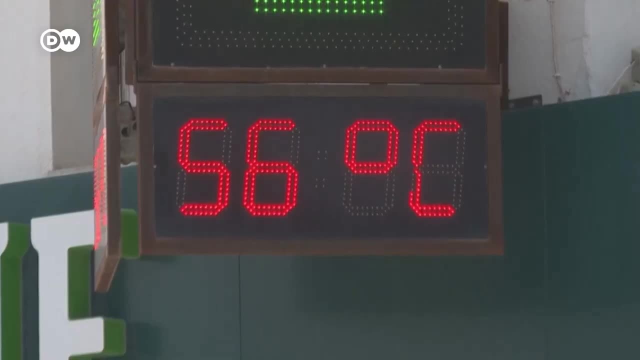 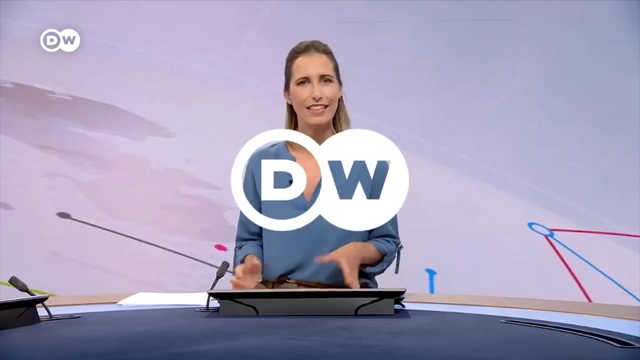 But superimposed to this warming, there are oscillations, there are fluctuations. One of those fluctuations is exceptionally high solar activity. The other is a warm weather phenomenon called El Niño. Translated from Spanish, El Niño means the child or the boy. It sounds harmless. But it's not. Last seen in 2016, it led to the world's hottest year on record. 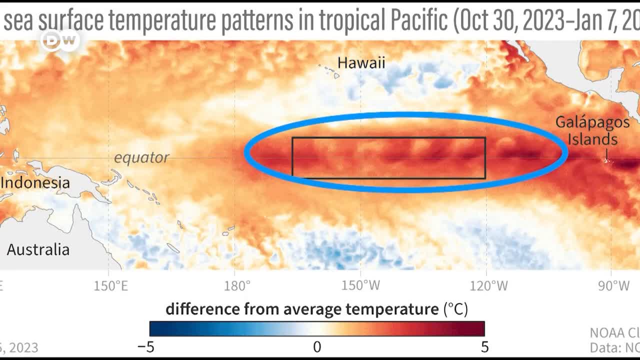 That's because El Niño impacts ocean temperatures which in turn affects the climate. 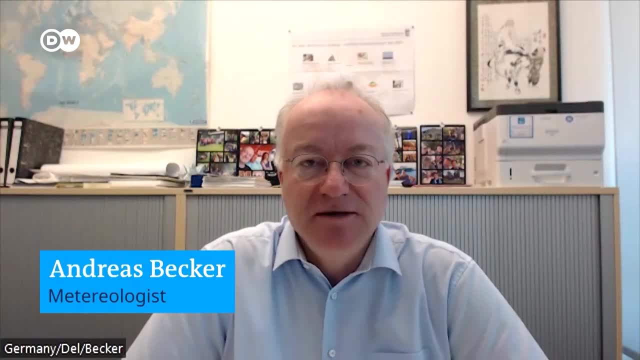 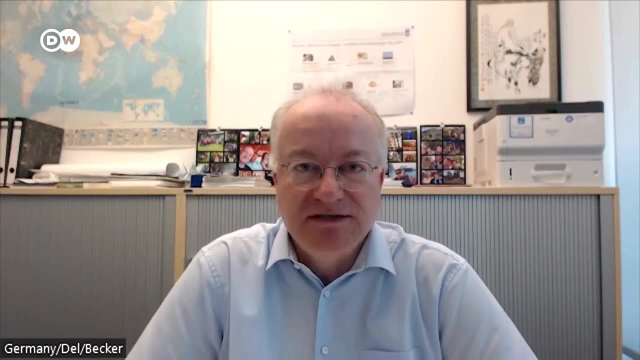 So the El Niño phase is also called the warm phase. Because as the upwelling of cold water on the coastline of South America and the Western Pacific is suppressed, the overall temperatures in the Pacific rise. 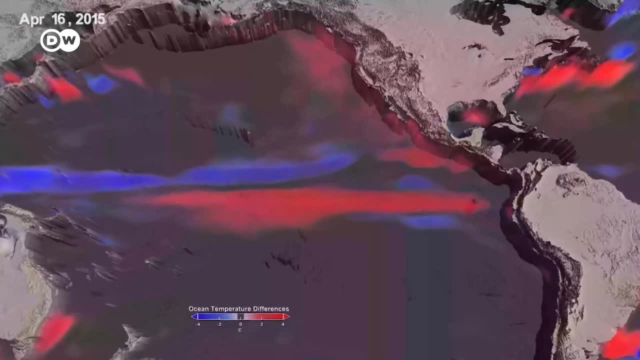 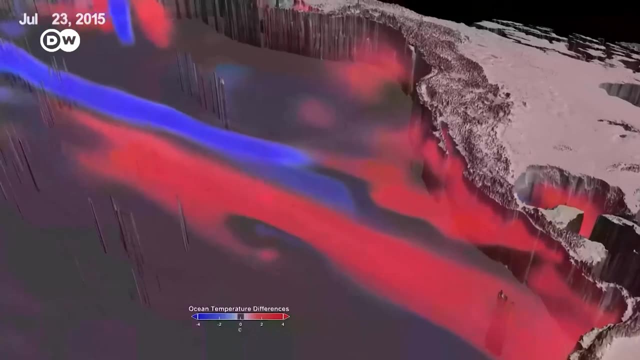 El Niño is a natural climate cycle and is associated with changing wind patterns and higher water temperatures in the East Pacific. So basically the ocean off the coast of Ecuador, Colombia and Costa Rica. 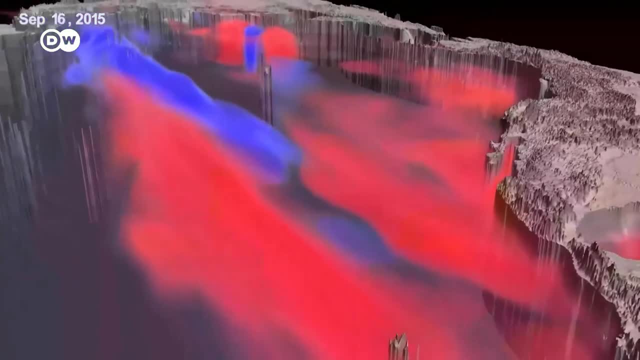 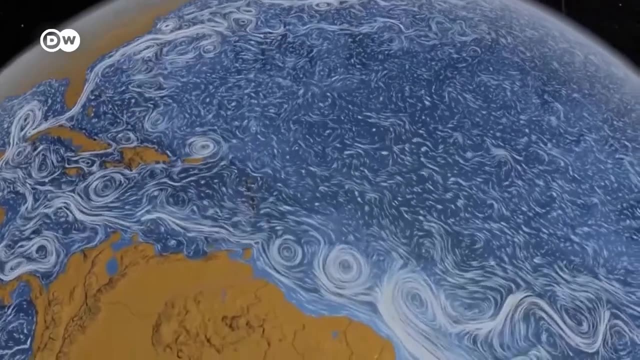 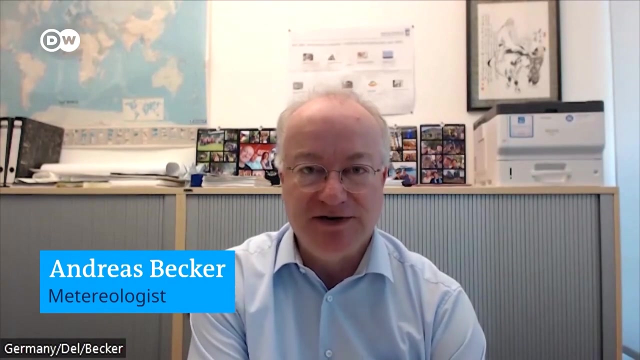 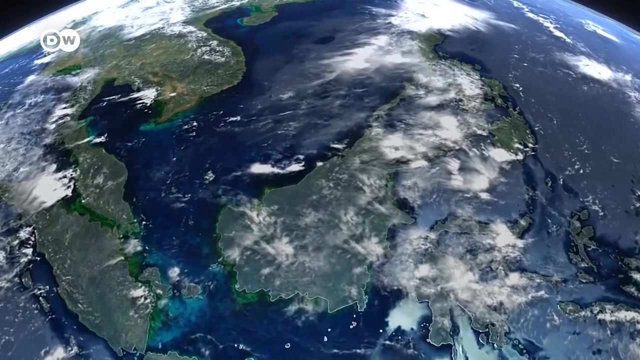 Here's another illustration from a previous El Niño event. Warmer waters just several degrees above average temperatures in the region influence ocean currents and weather patterns in large parts of the world. All of a sudden the rather wet areas in Indonesia and Australia have a dry anomaly. And in South America you have very wet conditions in areas that are normally very dry. And with these patterns there's also extreme weather conditions. And also extreme weather are related. And higher temperatures in the atmosphere. How much warmer it will get during the current El Niño is still unclear. 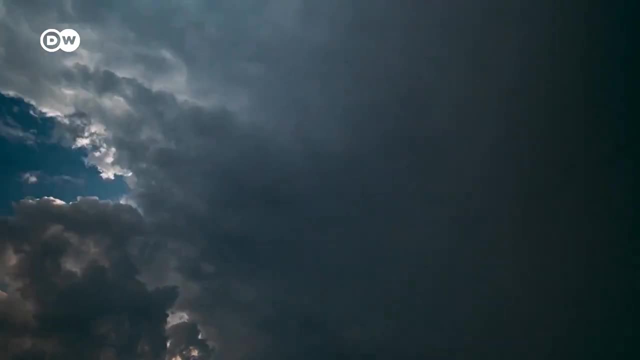 The good news, the phenomenon is expected to end by spring this year. But is that a reason to relax? Unfortunately not. 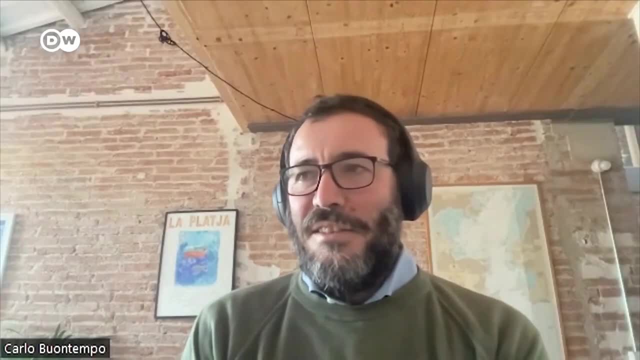 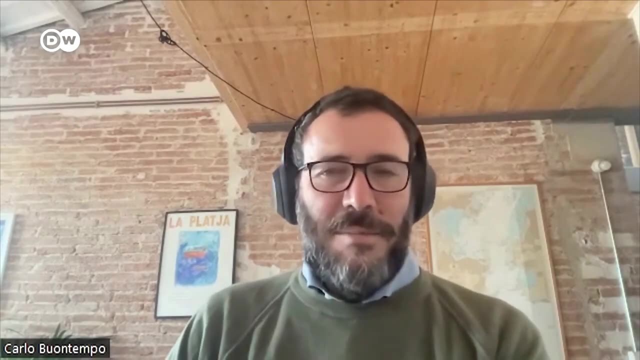 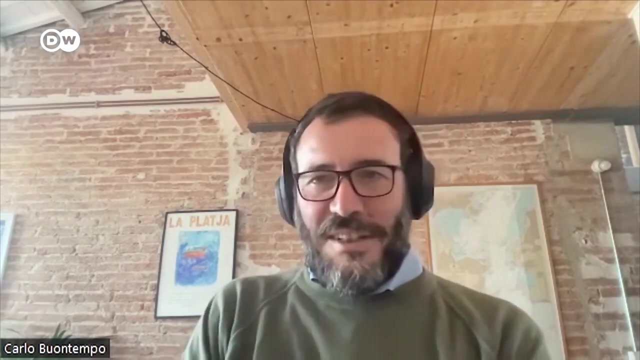 An analogy I like is like a ball rolling down a slope. And that's the climate change. The ball keeps going down because there is a slope. And then on top of this slope there are stones and holes and branches or things that may affect the trajectory of the ball. And so the ball bounces around in different directions. And that's the El Niño, the variation in the solar input, the volcanic eruption or all the rest. 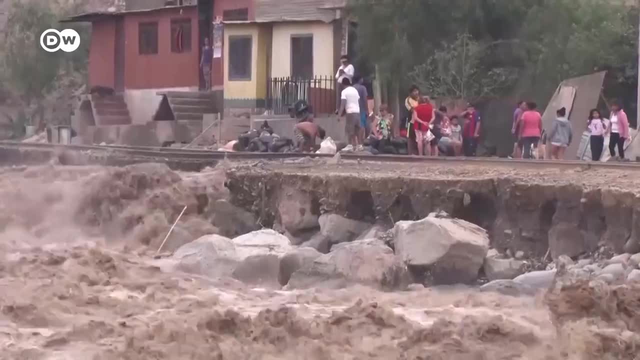 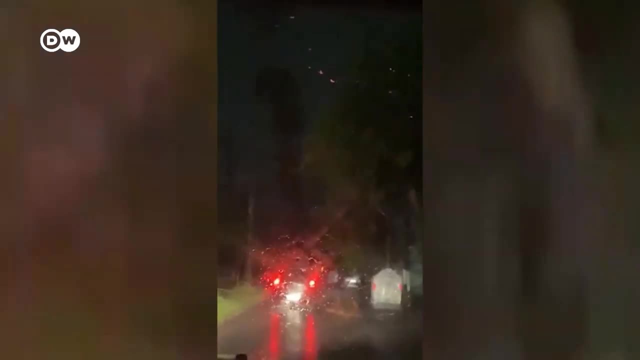 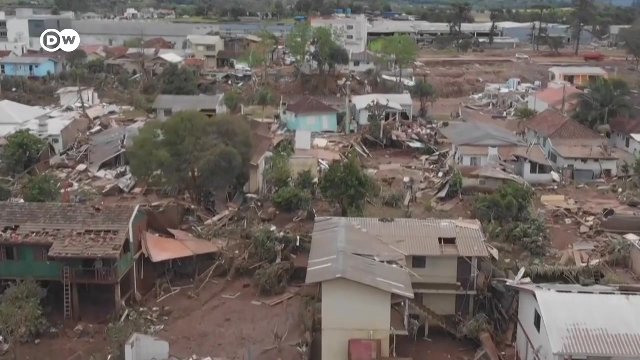 But still, after a while, the ball will be farther down the slope. Floods in Pakistan, wildfires in Croatian tourist centers last year, heavy storms in Brazil in January, heat waves around the world. Weather extremes linked to planetary heating are already causing catastrophic damages to lives and economies. 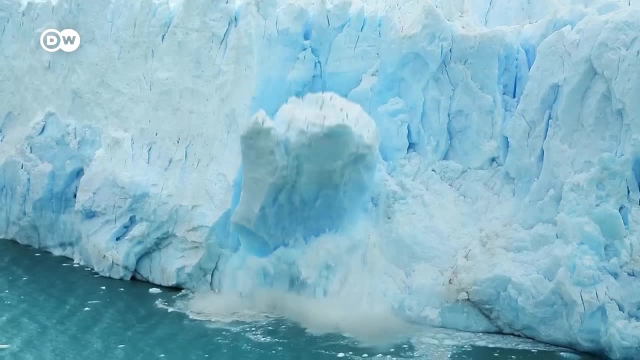 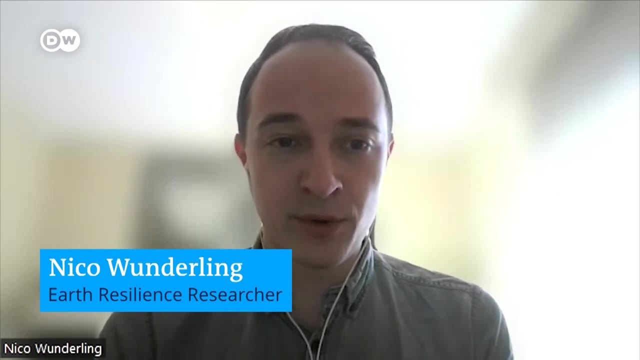 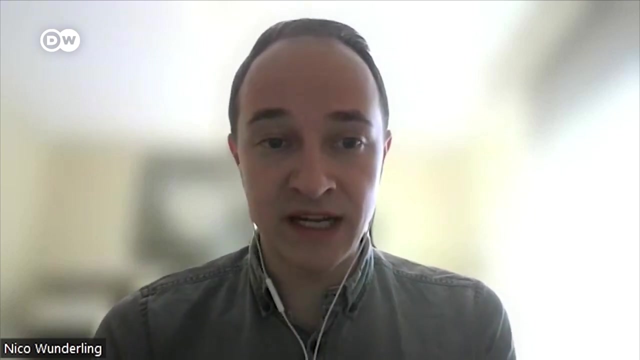 And that's all on top of bringing the planet closer to climate thresholds that trigger rapid and probably irreversible changes. I call them critical organs of the Earth that are important for planetary stability as a whole. And examples for tipping elements are the Greenland Ice Sheet, which has approximately seven meters of sea level rise. 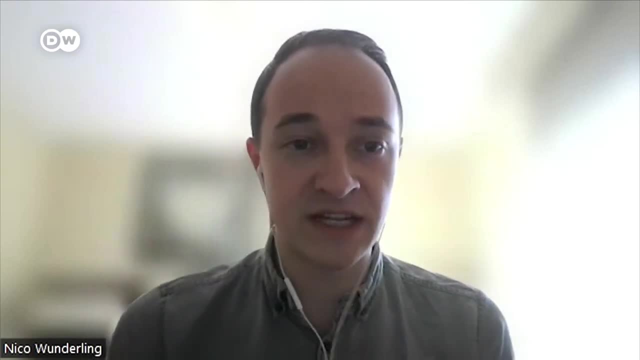 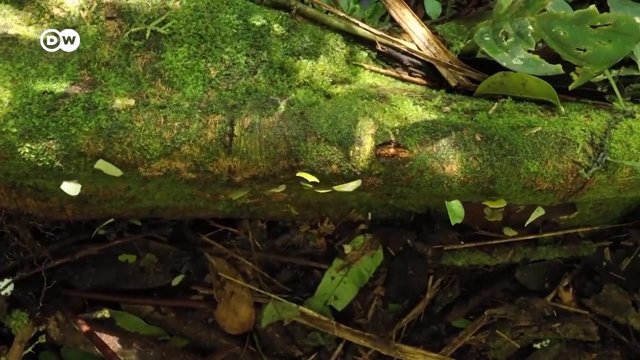 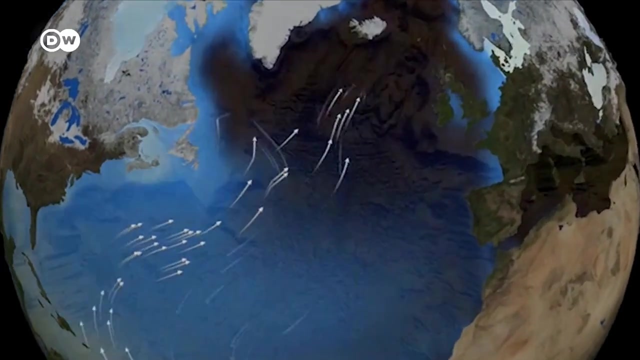 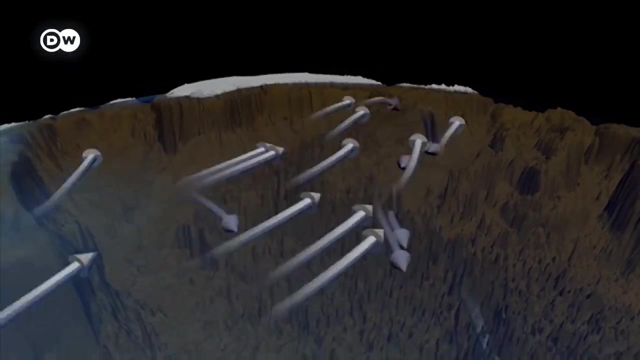 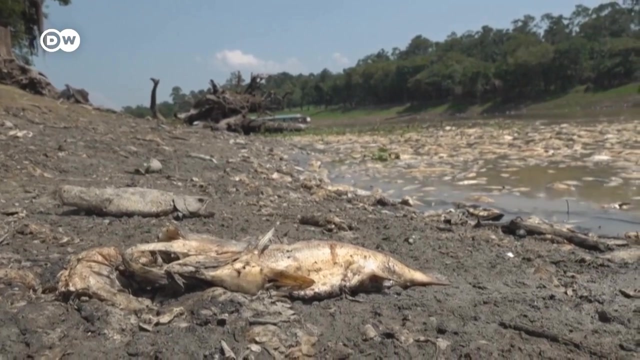 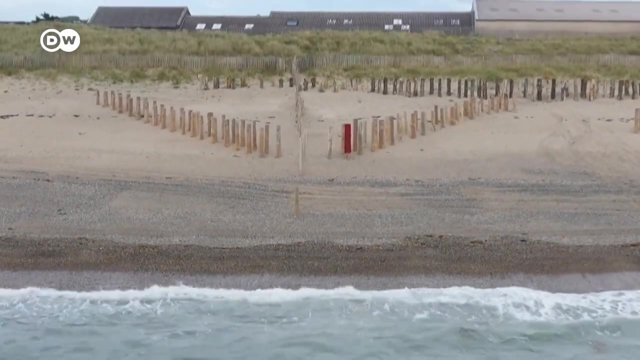 The West Antarctic Ice Sheet, which has between three to five meters of sea level rise if melted down. Other systems in danger to tip over are coral reefs and the Amazon. Recently, scientists expressed alarm over the latest findings that the so-called AMERC, a system of ocean currents in the Atlantic, is about to shift due to rapid ice melt. If it were to fail, Europe would see a dramatic drop in temperatures of up to 10 degrees on average. In Southern Hemisphere countries, warming could intensify and in the Amazon region, the rainy and dry season could be reversed. Sea levels would rise at a speed that would make it impossible for humans to adapt in time. So all these systems are now showing signs of a beginning instability. 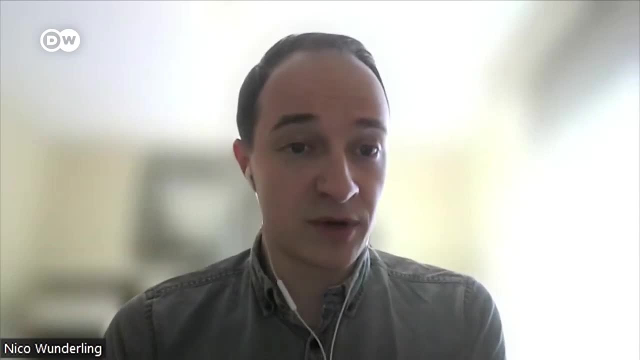 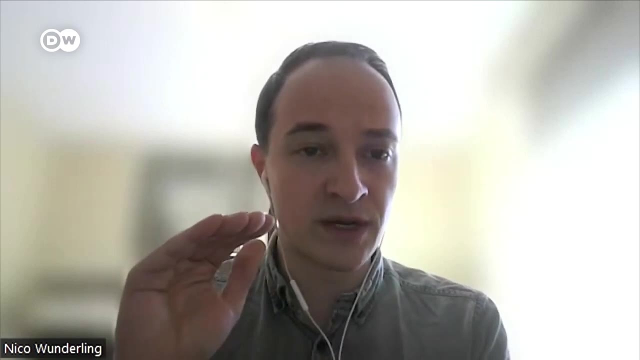 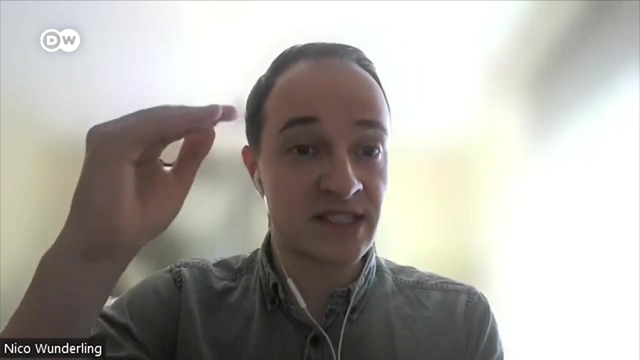 And that warns us basically that we should stop global warming as soon as we can and then get back to safe temperatures, which are on the order of long term, on the order of one degree. And the higher we get above 1.5 degrees, which is really a physical limit, the more or the higher the risk is that we lose some of these elements.